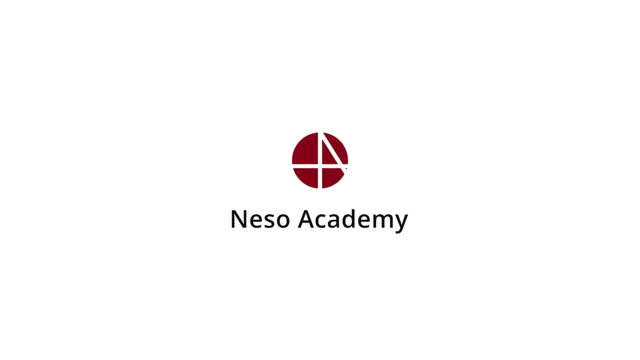 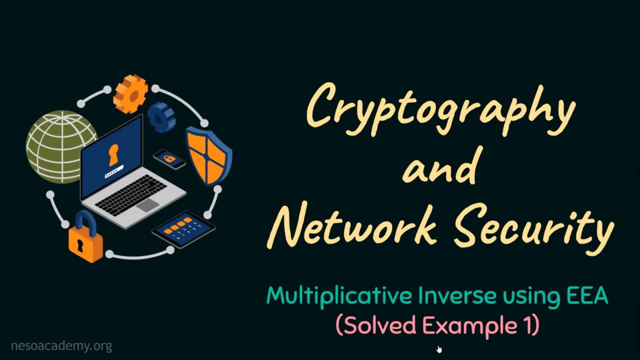 We have seen the basics of multiplicative inverse in the last presentation. In this presentation, we will focus on finding the multiplicative inverse using extended Euclidean algorithm. Let's see solved example 1.. While solving this example, we will understand how this extended Euclidean algorithm works. As usual, let's start the session with the. 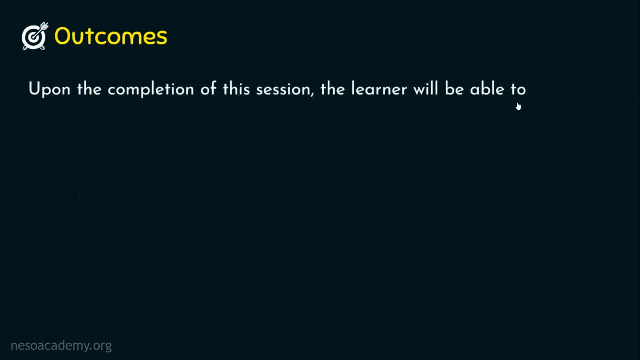 algorithms. Upon the completion of this session, the learner will be able to Outcome: number 1, we will know about multiplicative inverse and outcome. number 2, we will determine the multiplicative inverse of a given number under mod n using extended Euclidean algorithm. 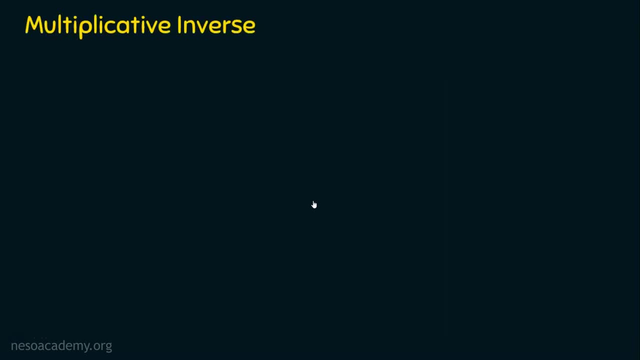 From the last presentation we understood what is multiplicative inverse and we also have seen how to find multiplicative inverse manually for smaller numbers under modulus. So when small numbers are given, it's easy to find the multiplicative inverse. Think if the number is a big number. Obviously we need some algorithm, right? 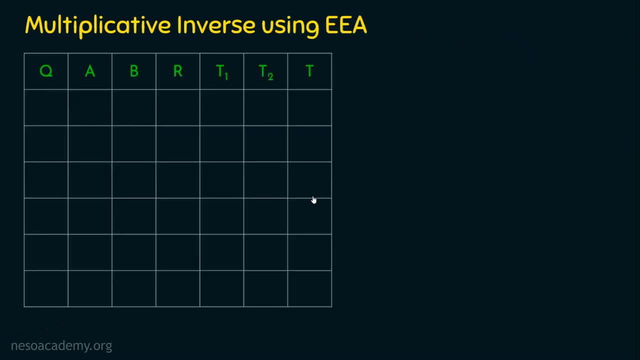 For that we are going for the extended Euclidean algorithm. So we are here to find the multiplicative inverse using extended Euclidean algorithm. Now, if you see here I am gonna explain this in the tabular column approach. Just recollect the lecture: finding GCD, method 1.. 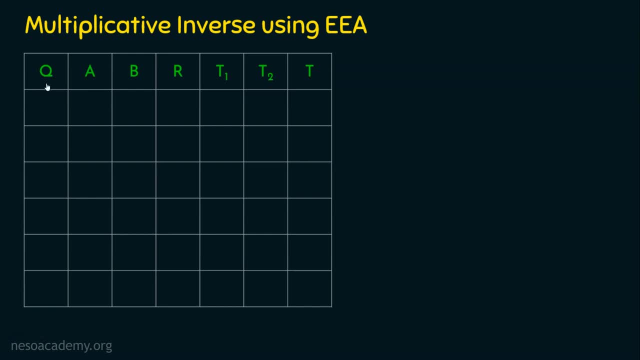 In method 1, what four columns we had. The first column is the quotient, then a, b and the remainder. So we had only these four columns when we solved some problems using Euclidean algorithm. To be precise, method 1 of Euclidean algorithm. 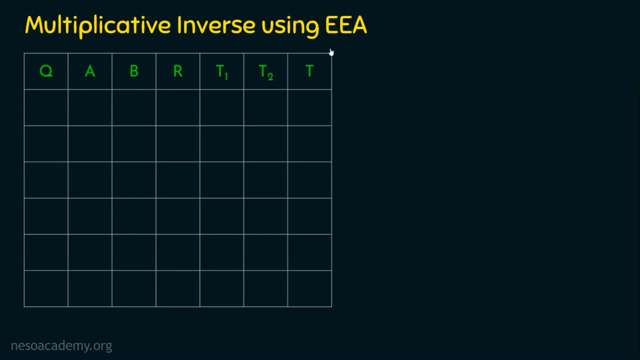 Now we are going to extend this Euclidean algorithm And that is why it is named as extended Euclidean algorithm. What is the extension we are making? We are additionally including three more columns: t1,, t2 and t. Don't worry about all the columns. 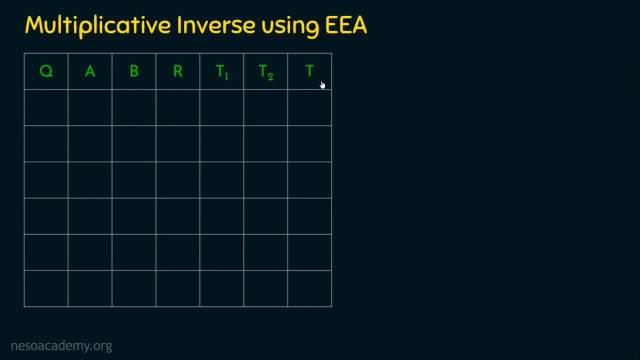 Anyway, when we solve the example problem, we will understand things clearly. Now, as usual, we have a set of prerequisites. Let's start. The points to ponder include. the first point is: a should be greater than b, And we are very well aware of this because already while solving the problem of GCD, 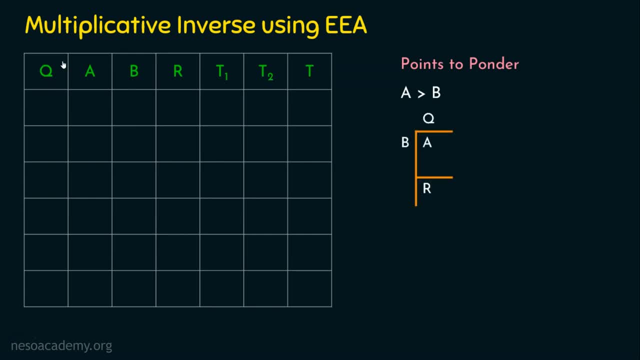 we understood that a should be greater than b And we know how to fill this q and r. So, after placing the values of a and b, we know how to fill the values of q and r. It's so simple: a mod b. we are going to perform. 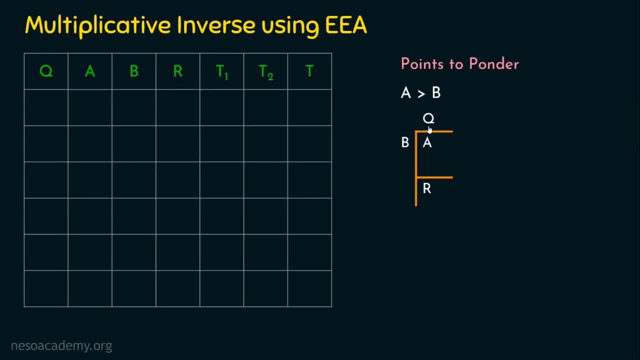 So we are going to divide a by b. Obviously, we will be getting some quotient and remainder. Quotient value will be placed here And the remainder value is going to be p. We are very clear about this because already we have seen this in the GCD method 1 using Euclid's algorithm. 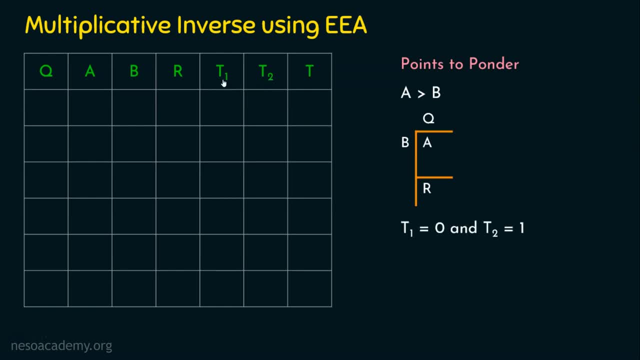 What are all the new things here? The new things here introduced are t1 and t2.. For the first iteration, or for the first time, t1 and t2 values are 0 and 1 respectively. So when you are dealing with the first row, place 0 in t1 and 1 in t2.. 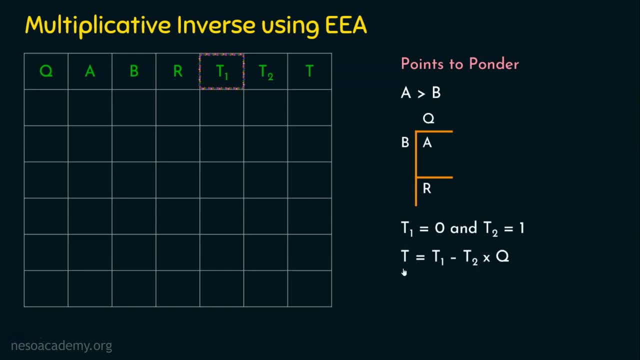 Then we are going to compute t. I'm just giving the formula for t: t is equal to t1 minus t2 into q. So you just use this formula, Don't worry about this. Anyway, I'm not going to explain how we get this, because we are going to just use this extended. 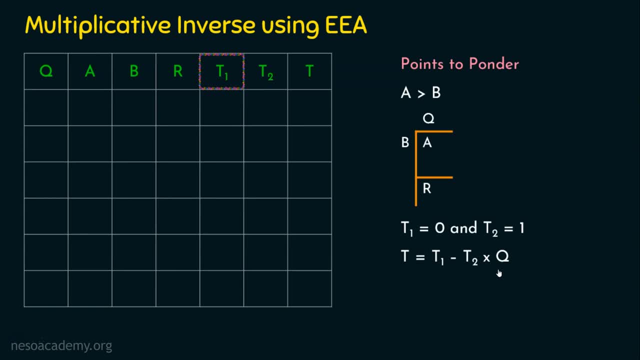 Euclidean algorithm to find the multiplicative inverse, and this is not a mathematics class, So just use this formula: t is equal to t1 minus t2 into q, So obviously the first row will be filled. right After completing the iterations, you will be encountering a situation where you cannot move further. 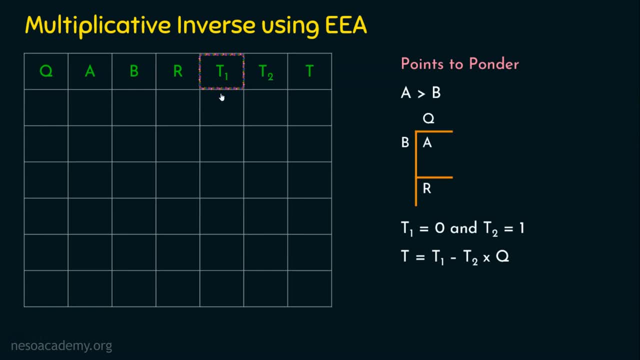 the algorithm further In that case. so whatever is there in t1, that is going to be the multiplicative inverse. I hope things are clear. If things are not clear, no worries. When we see the example, you will understand this easily. 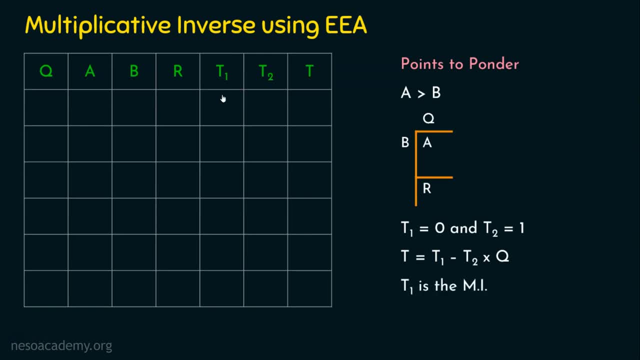 So, as mentioned, when you find a situation where you cannot proceed with the division further, then that moment. so whatever is there in t1, that is going to be the multiplicative inverse that you are looking for. So let's see the example now. 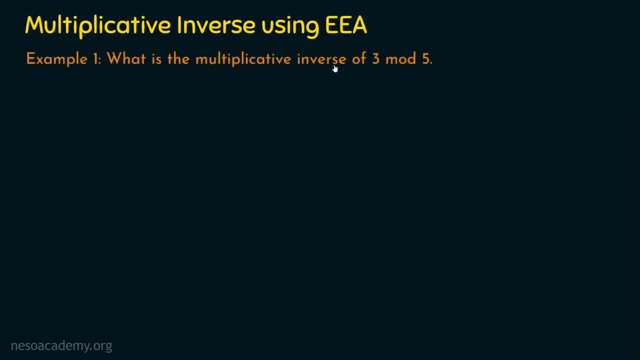 Example number one. This is the multiplicative inverse of 3 mod 5.. As already mentioned in the previous lecture, there exists a multiplicative inverse only when this value and this value are relatively prime to each other. Since 3 and 5 are relatively prime to each other, we can definitely say there exists. 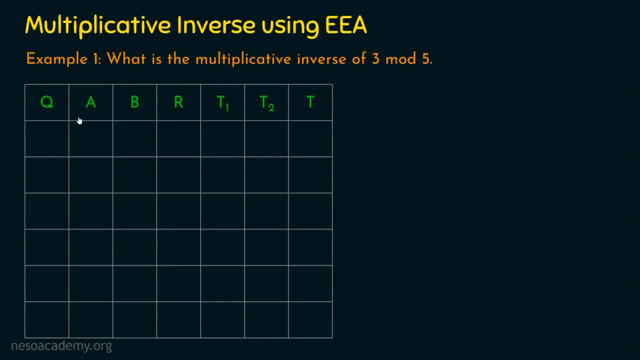 a multiplicative inverse. Let's solve this now. We know the solution includes seven columns- q, a, b, r, which we had in the Euclid's algorithm way of computing GCD, And we are extending this Euclid's algorithm like. 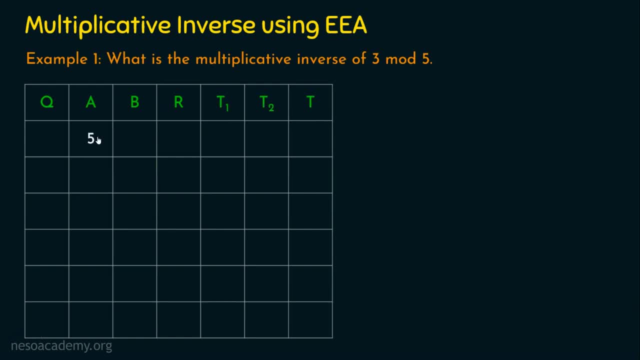 t1,, t2, and t. As already mentioned, a should be taking the bigger value, right. So 3 and 5, what is the bigger value? 5.. So 5 is placed in a and 3 is going to be placed in b. 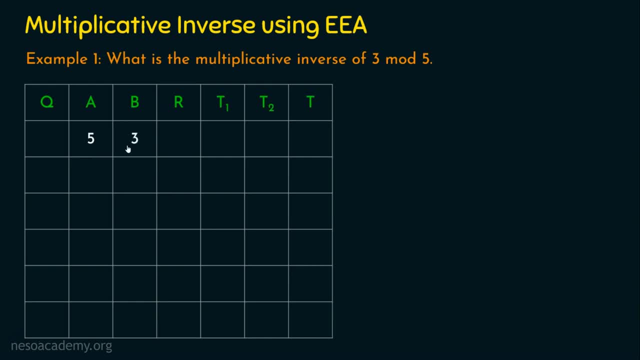 Now we are going to do the simple computation, that is, the division operation a mod b. When we perform a mod b, 5 divided by 3, 3, 1 times 3, and the remainder is 2.. So we are just going to fill this quotient, in which place? 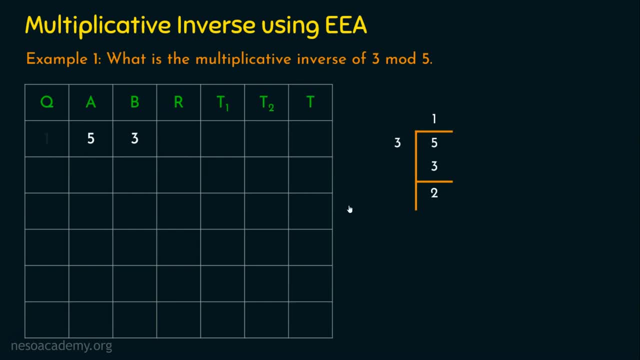 This place And this remainder in this place, right? So we are going to fill 1 in the quotient and 2 in the remainder. Now, as already mentioned, for the first row, the value of t1 and t2 are set. 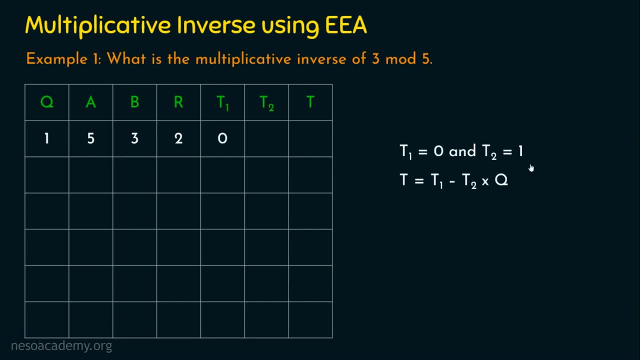 So t1 is equal to 0 and t2 is equal to 1.. So I'm just filling: t1 is equal to 0 and t2 is equal to 1.. And we know how to compute t right? This is the formula. 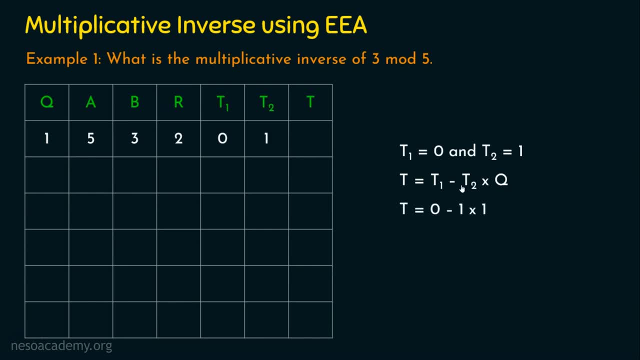 So when we use this, t is equal to t1, we know it is 0.. t2, it is now 1.. So 0 minus 1 into 1.. So when we evaluate this, we get 0 minus 1.. 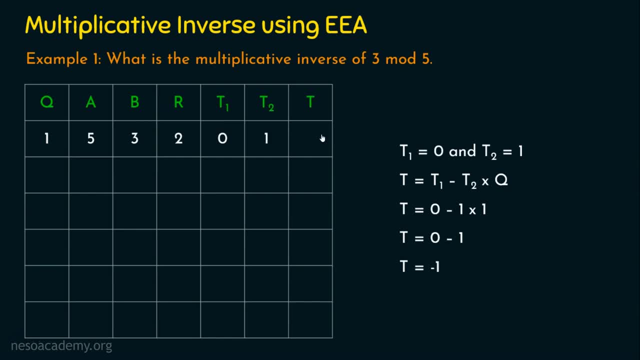 Finally, we get t. t is equal to minus 1.. I'm going to take and place this value here. So we get: t is equal to minus 1.. So first row is over. Then what we need to do? Just recollect what we did in Euclid's algorithm. 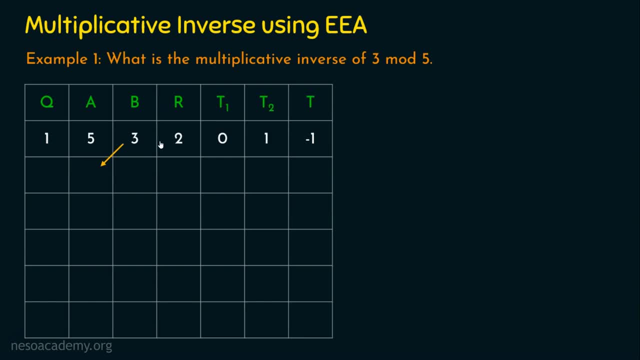 We did shifting operation right. So the same shifting we are going to perform. Whatever the value of b, that is going to be stored in a. whatever the remainder is, that is stored in b, right? So the value of b is shifted to a and the value of r is shifted to b. 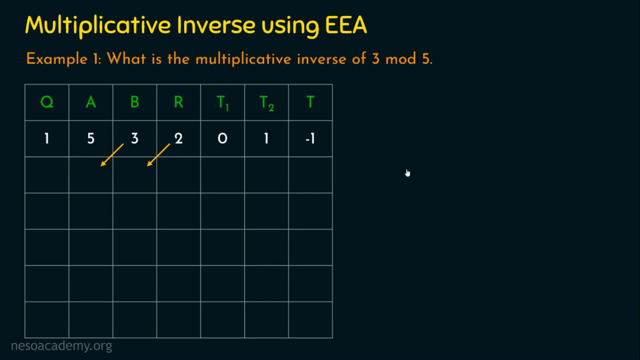 We did only this in Euclid's algorithm, But we are going to do something additionally here, which is the value of t2 is placed in t1 and the value of t is placed in t2.. So, if you remember this, that's it. 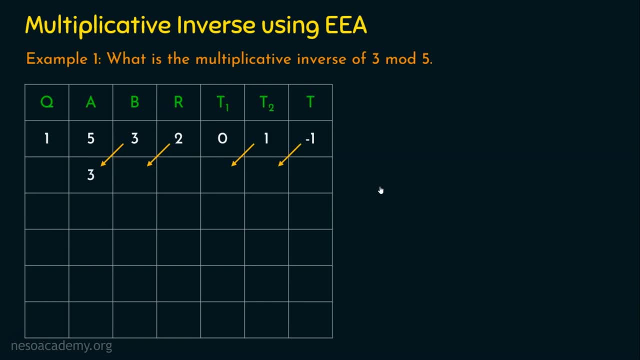 You can easily solve this problem Now. a is going to store 3.. b is going to store 2.. t1 is going to store 1 and t2 is going to store minus 1.. So now repeat the algorithm, What we are going to do. 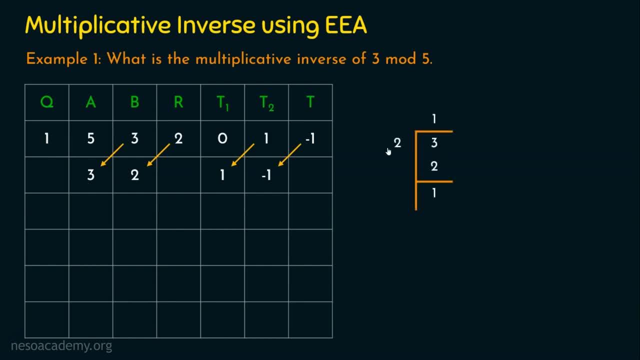 Do a mod b right. When you do a mod b, 3 divided by 2.. 2, 1 times 2.. The remainder is 1.. Here quotient is 1.. Reminder is 1.. So quotient is 1 and remainder is 1.. 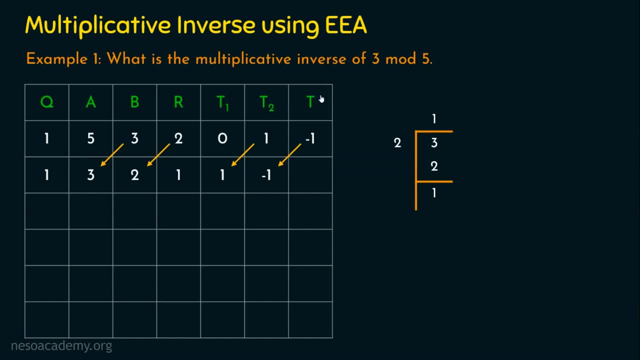 I have completed filling this detail. Now we are going to compute the value of t For this. we are not going to take 0 and 1 for t1 and t2 respectively, because this is only for the initial condition. Now we have the value of t1 and t2, right. 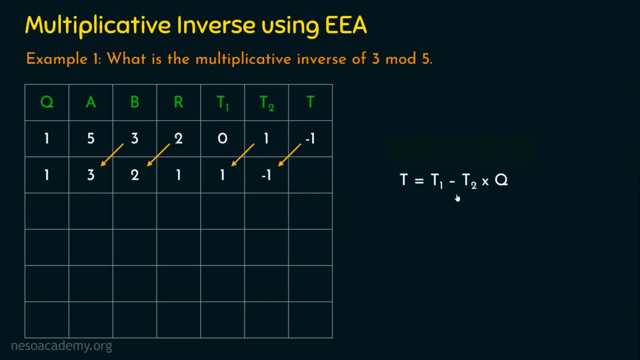 So we are going to use this value Now. we are going to take this formula and apply what's the current value of t1.. It is 1, right? So t1 is 1 minus t2.. t2 is minus 1 into what is q. 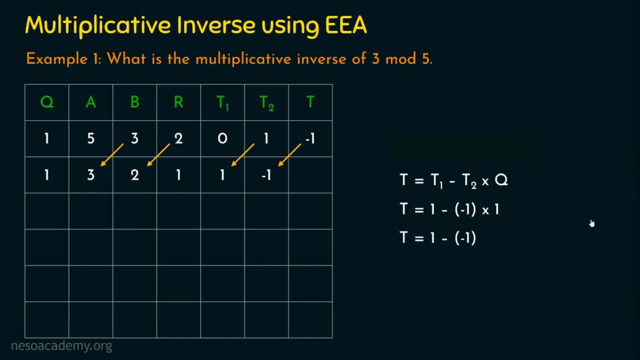 q is 1.. So I am taking this value. When you evaluate this, you get t is equal to 2.. I hope things are clear. So I am just going to take this value. I am going to place this here. So I am just filling 2 here. 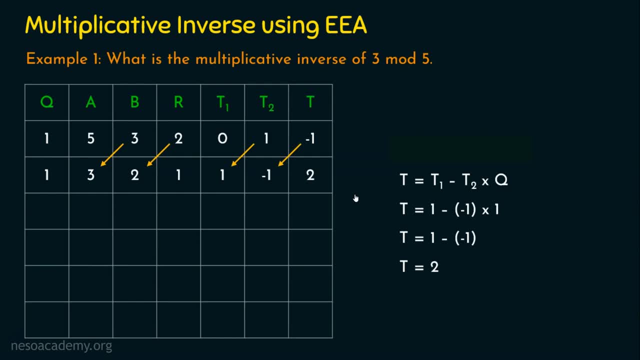 So the second row is also filled. Are we able to proceed with the algorithm? Yes, let's see So what we are going to do, We are going to do the shifting operation. Let's start the shifting. So a takes this value and b takes this value right. 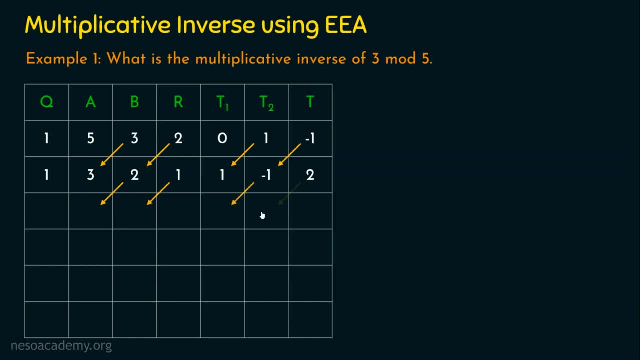 Similarly, so t1 takes this value And t2 takes this value. So let's fill the values. So 2, 1, minus 1 and 2 are taking their respective places. Now let's run the algorithm again. We are going to do a mod b, right? 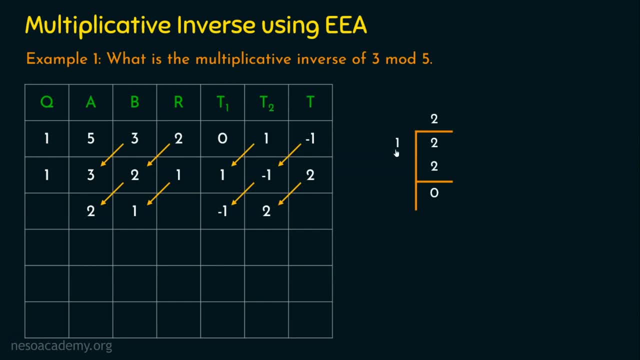 So 2 mod 1.. So when you perform 2 mod 1, you get 1, 2 times 2.. The remainder is 0.. The quotient value is 2.. The remainder is 0.. And what about the t value? 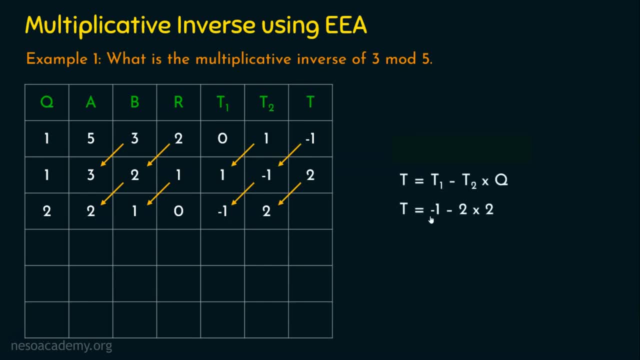 Where t1 is minus 1 and t2 is 2.. So just apply this value minus 1,, 2 and 2.. Why this 2? Because the quotient value right now here is 2.. I hope things are clear. 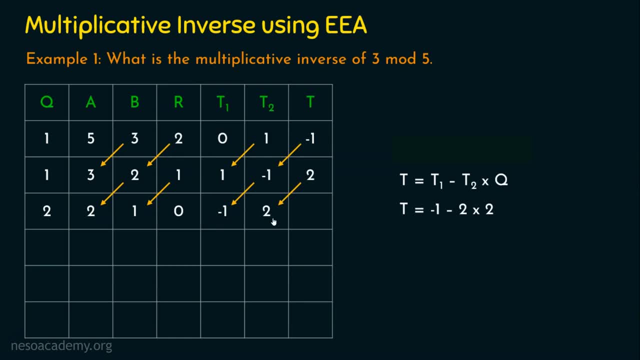 t1 is minus 1.. t2 is 2, because this is t2.. And what about q? here q is 2.. So we are just substituting the values and evaluating this. We get t is equal to minus 5.. 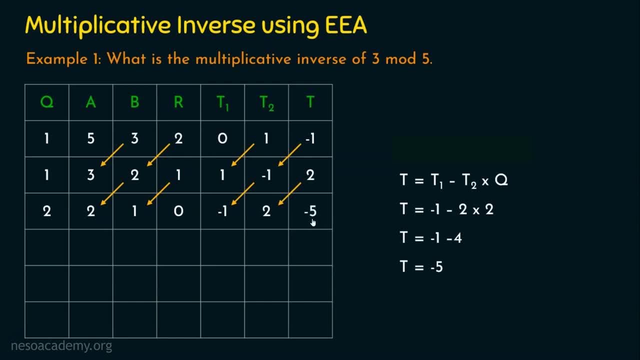 I'm just placing this value in the appropriate place. So third row is also complete. Let's proceed with the algorithm further. So whatever is there in b, it is assigned to a. Whatever is there in the remainder, it is assigned to b. 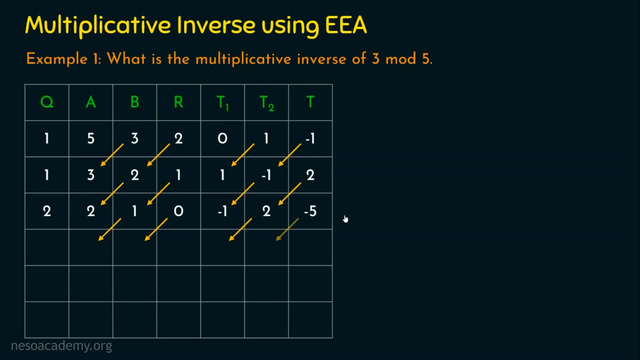 Similarly, we are going to do the same thing. Whatever is there in t2 is given to t1. And whatever is there in t is given to t2.. Let's shift the values now. 1 is taking this place. a now has 1..